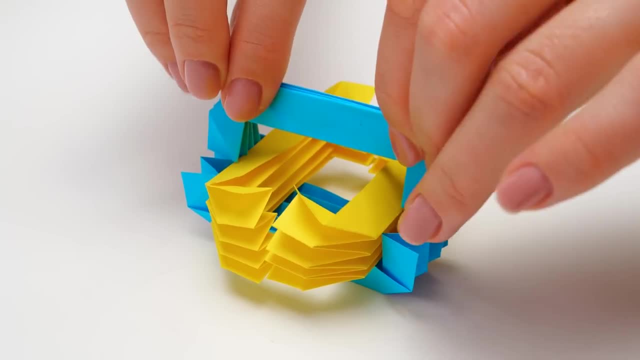 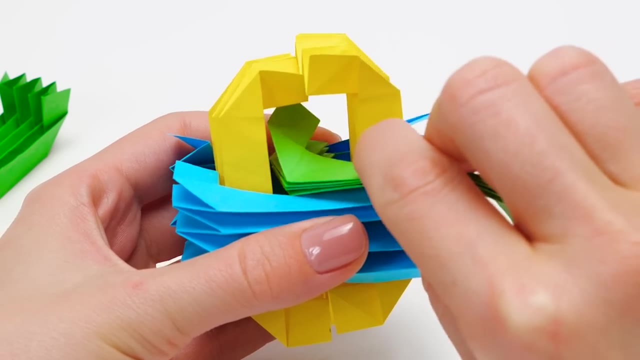 First step. Now these go like this, And then this one goes on top. Yeah, it's a bit tricky, I know, But I'm sure you will love the result. That's the cube we've got. What do you say, Sammy? shall we play? 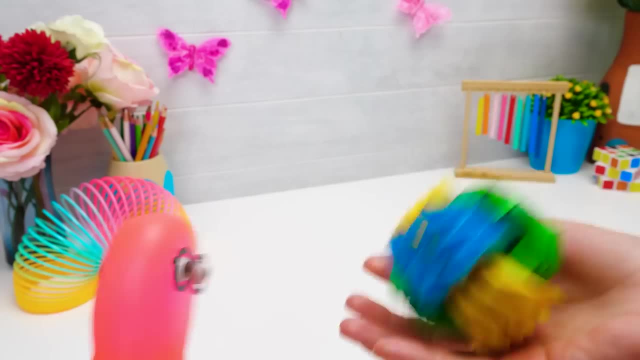 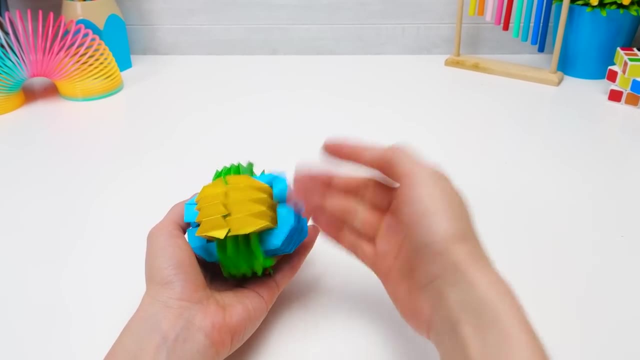 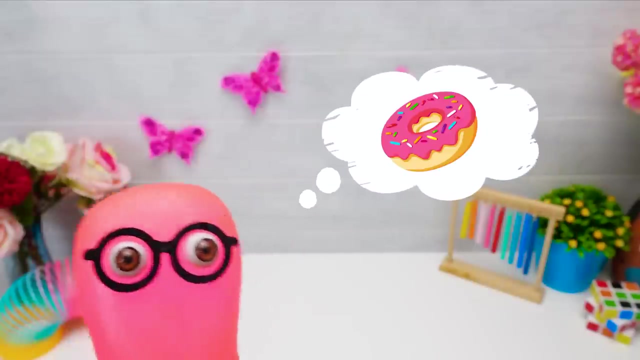 Whoa, This looks so much fun. Oops, I think I'm hungry. Yeah, I could eat something too. You know, this gave me an idea for our next craft. We need to make a nice cake, No Better. a craft with candy. No, No, A donut. 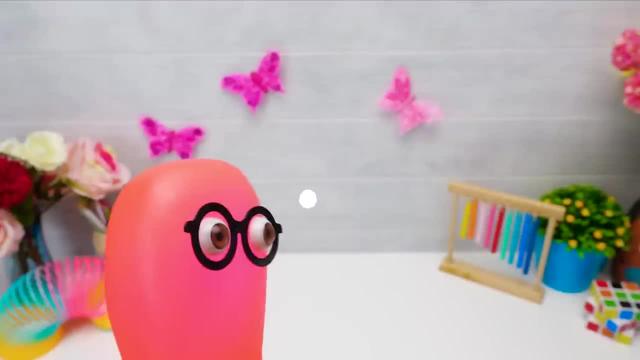 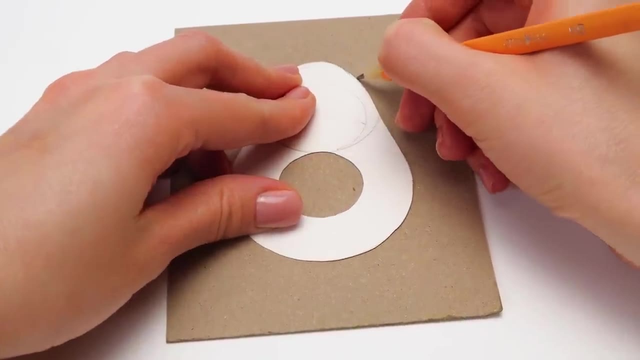 Yeah, nice, try Sweet Tooth. We're going to make an avocado pop-it. What? No candy. That's not fair. I'm sorry. It's just that avocado is so cute I couldn't resist. Alright, then, I support cuteness. 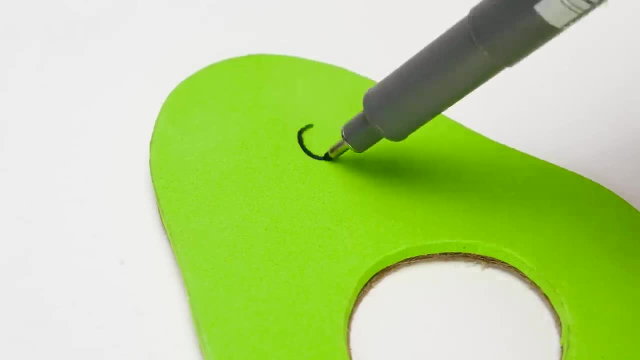 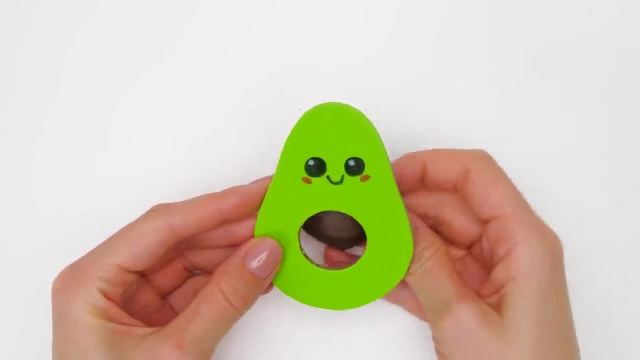 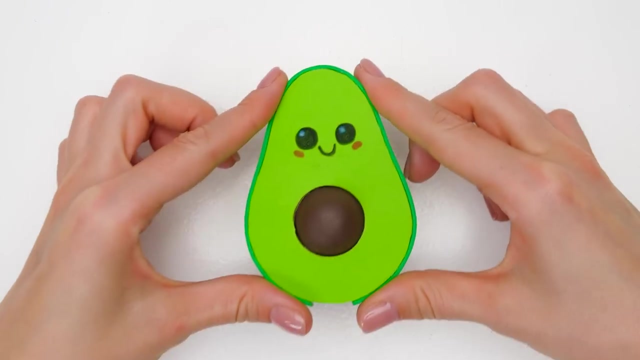 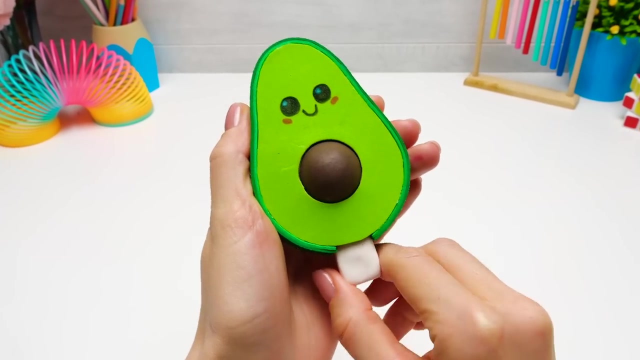 Awesome. I'll even take part in making this avocado even cuter. Oh, that's so sweet. Great job, Sammy. Now let's put it all together. Here we go. It should look nice and neat. Well, what do you say? 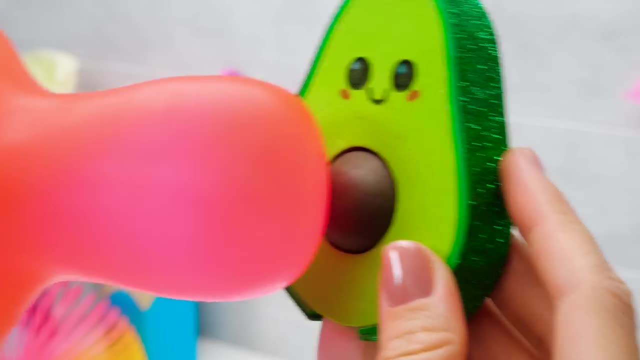 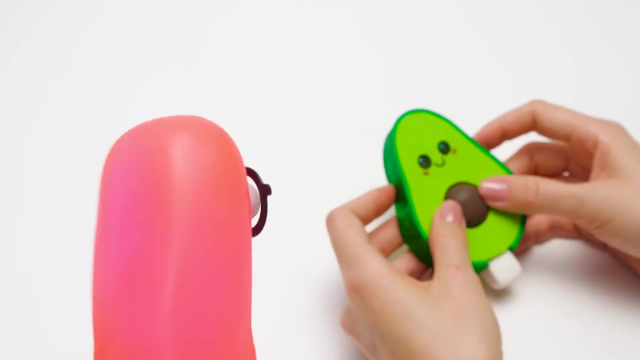 Wow, Let me poke a pop-it too. And the best part, our pop-it works as an eraser as well. Huh, I'm so hungry. What if I just take a tiny bite? No, Sammy, you can't eat it, No way. 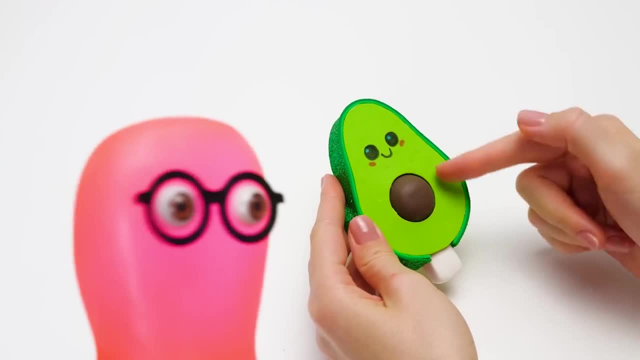 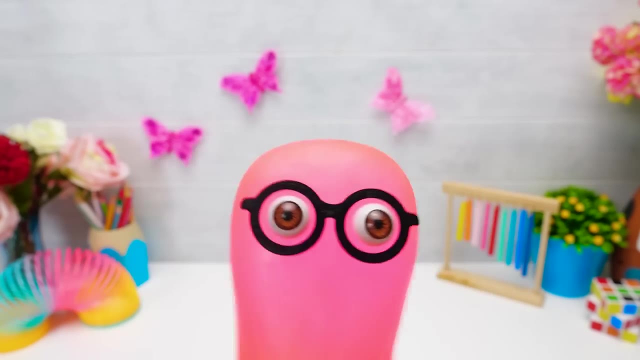 But I want to eat it. so much Wait, I know something to distract you. Huh, I hope it's something tasty, I mean inspiring, Or I'll start eating everything in my set. I promise you'll love it. Just give me a couple minutes. 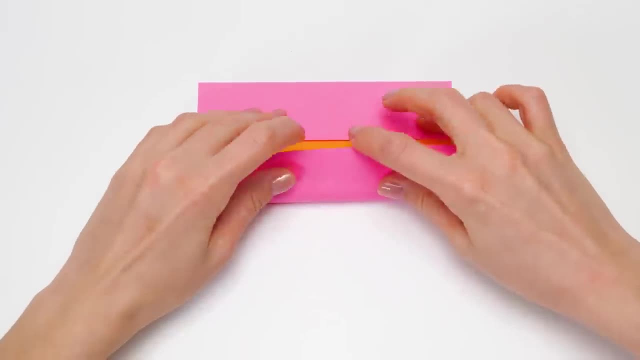 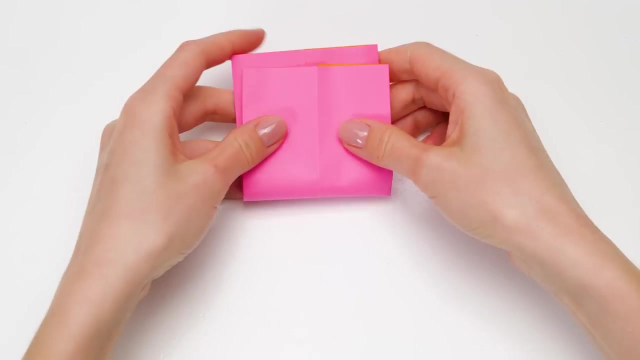 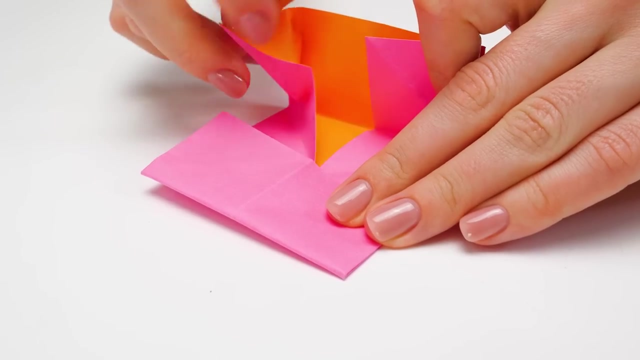 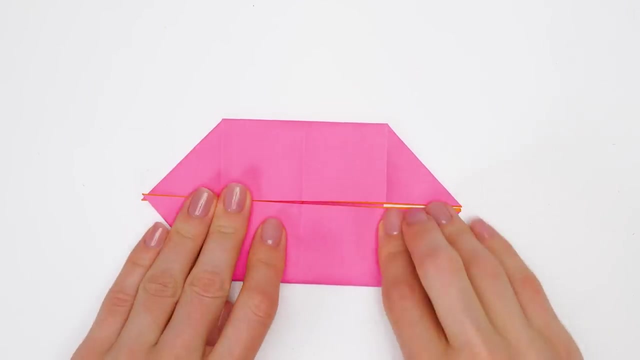 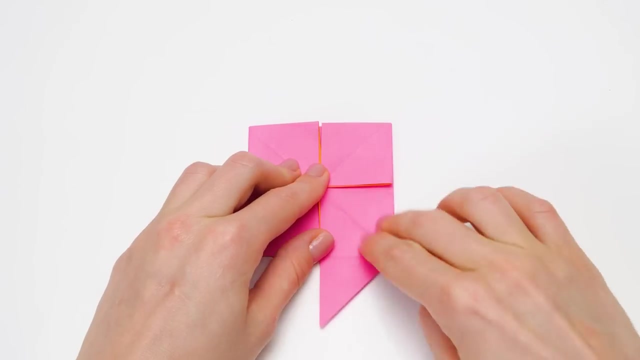 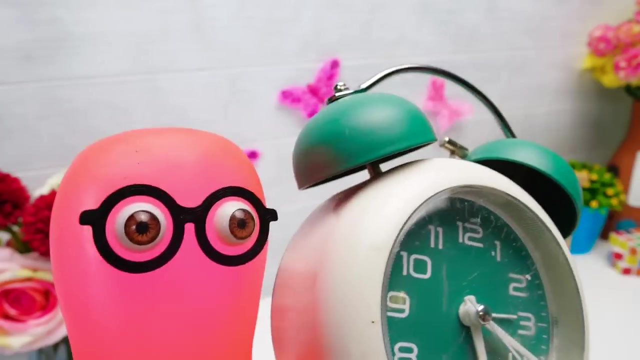 Two minutes Clock's ticking. What Am I on time now? Okay, Time's up. Too bad, you didn't make it. I'm starting to eat everything in my sight Right now. Hey, Stop fooling around. Why don't you better find me a marker? 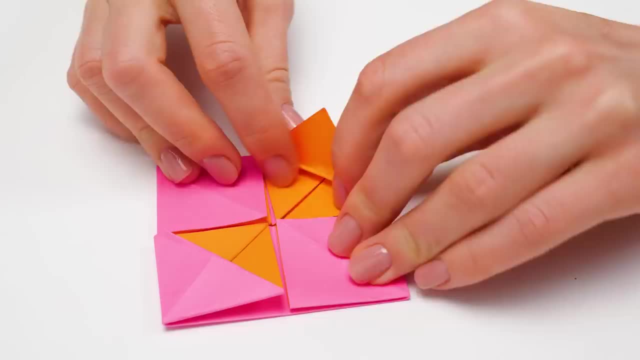 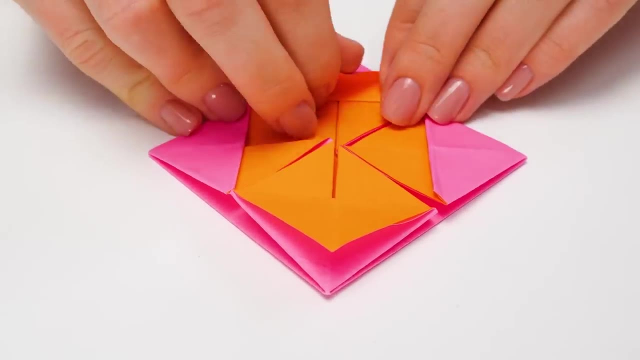 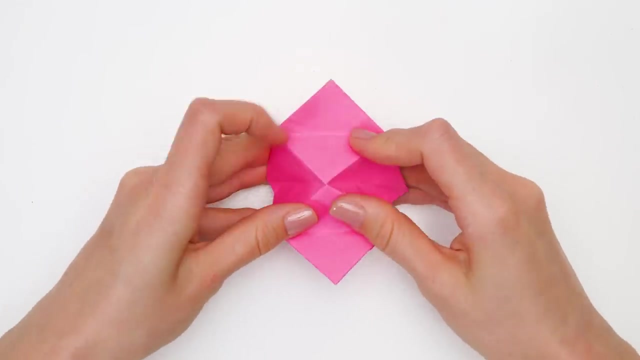 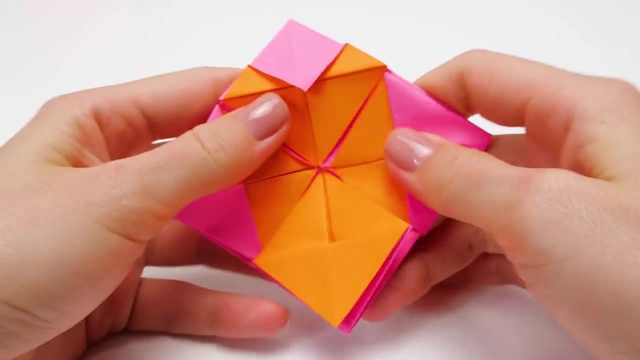 I'll get you a marker. Here's a marker Ready. Let's add some light to this. look, We shouldn't break off the. Also, you need to Ship it. Here's another marker. Alright, here's a marker, But I'll get to draw the face. 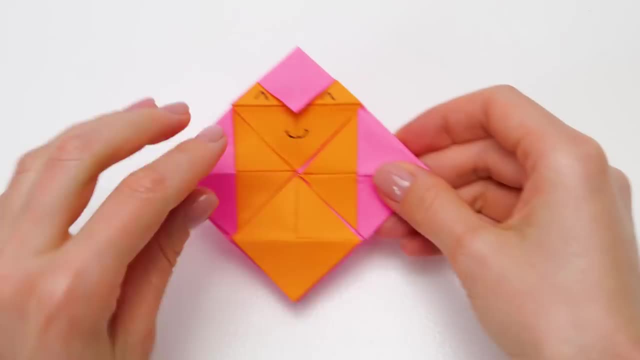 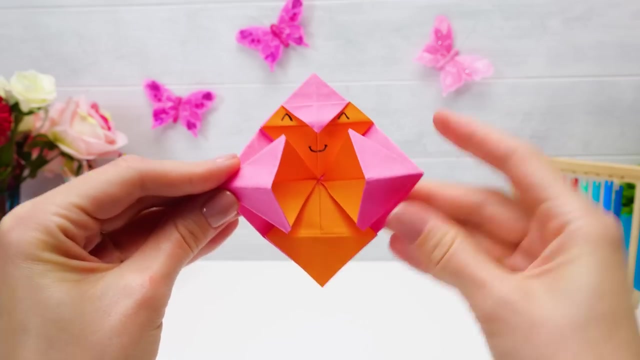 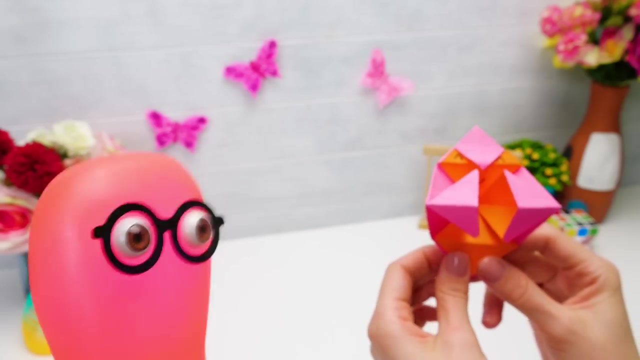 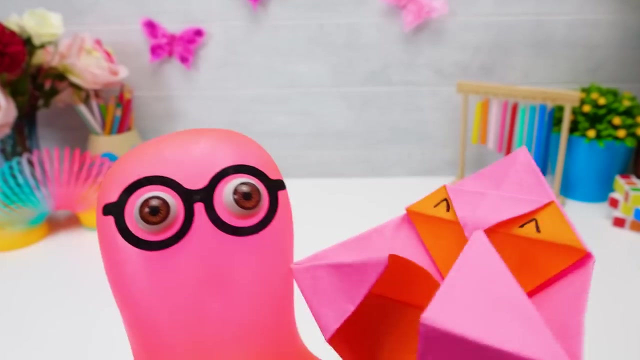 the face cute. let me only put the last pieces together and voila, this is a little monkey and she's having a good time. well, whoa easy tiger. although you were spinning so hard that now I want to put it on paper. we're going to make a. 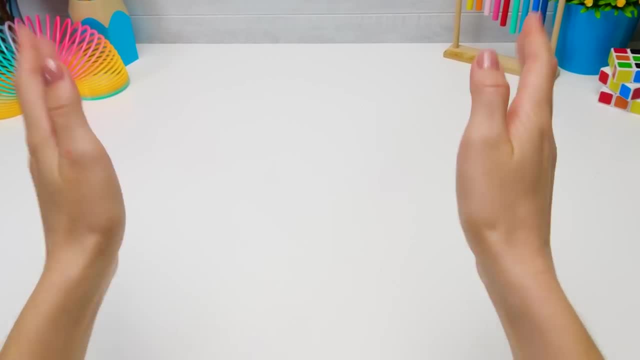 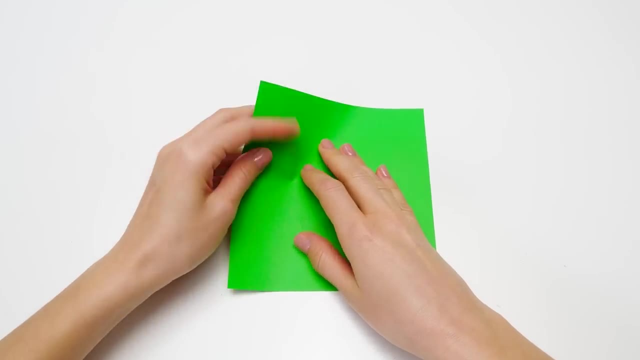 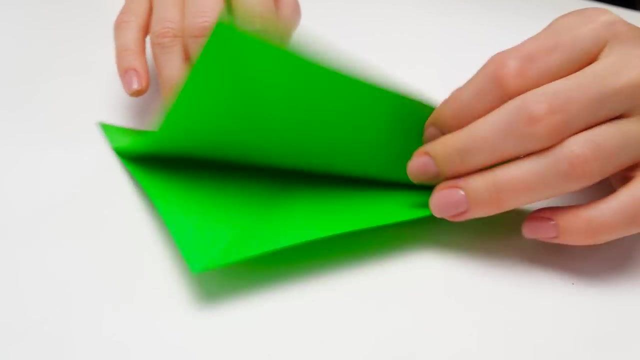 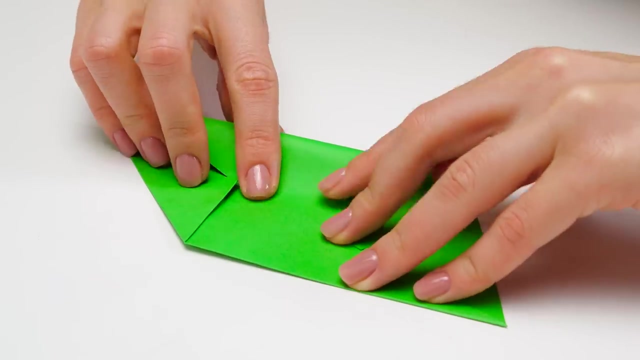 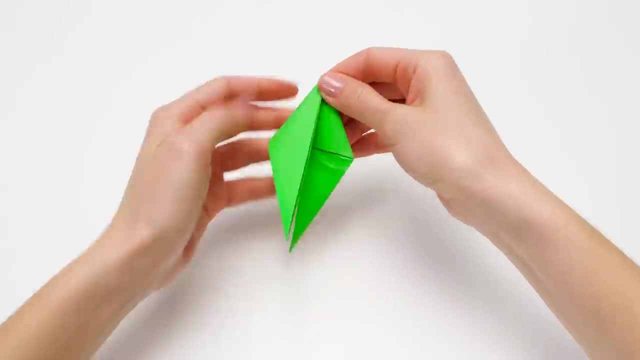 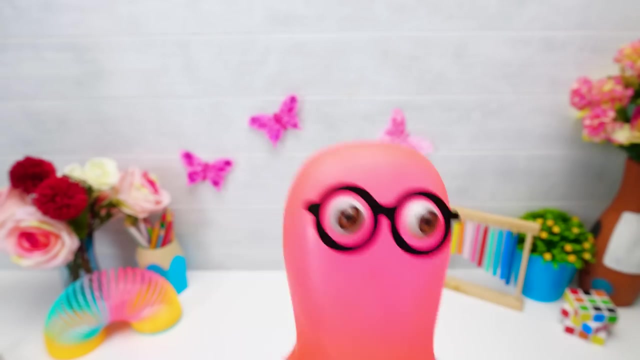 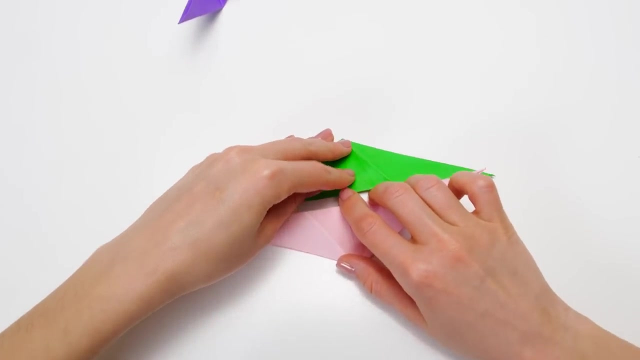 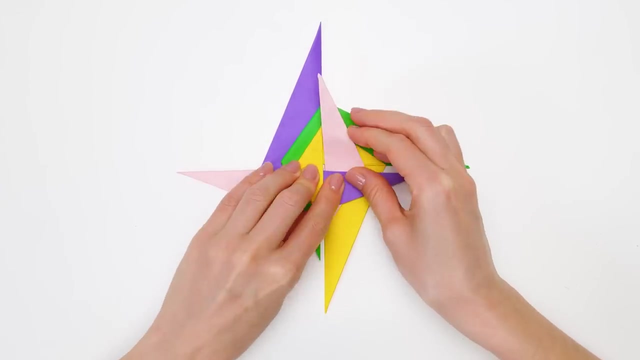 spinning top. for this we will need paper, of course. okay, now focus and make not one, but several sheets of paper in different colors at once. I'm trying to. it doesn't work. maybe I should spend harder. oh, Sammy, Sammy, I think you better lie down and you friends watch closely. 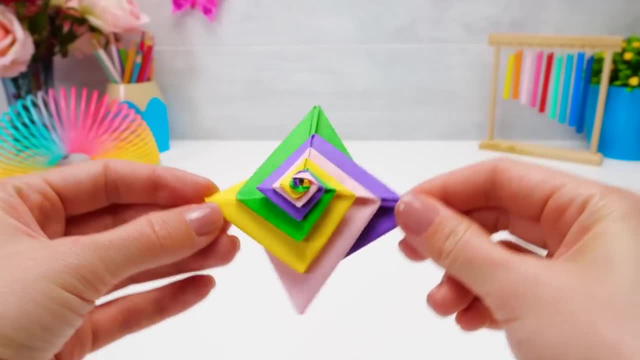 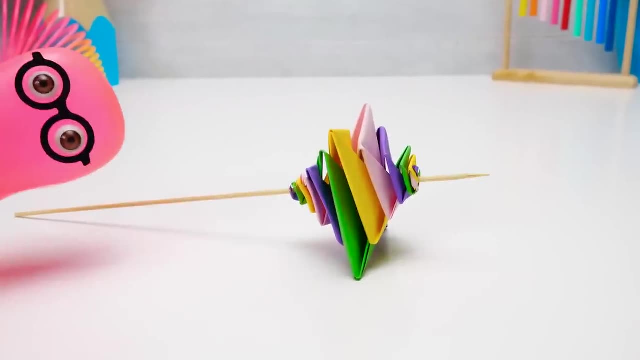 great, right, I need a wooden skewer or something and then I'm done, as always. Now, the moment everyone has been waiting for It's Sam's big throw. He did it. He really did it. Yay, The crowd's cheering, The fans are swooning. 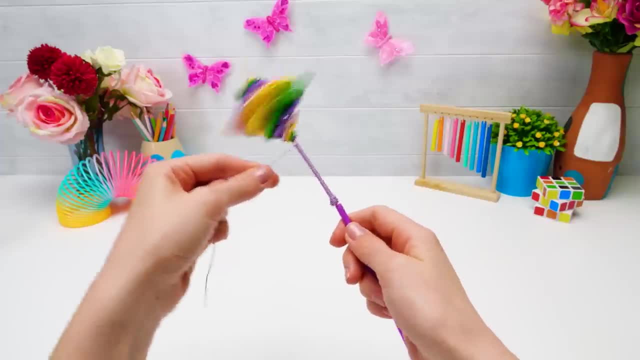 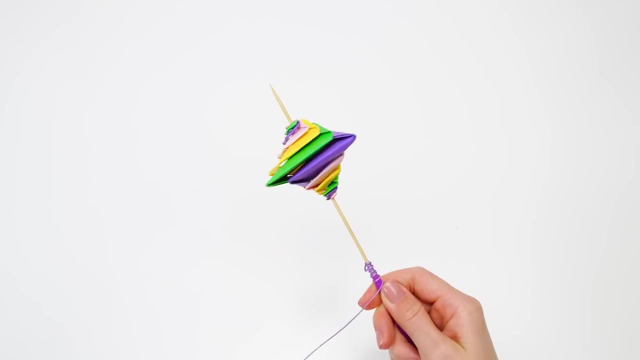 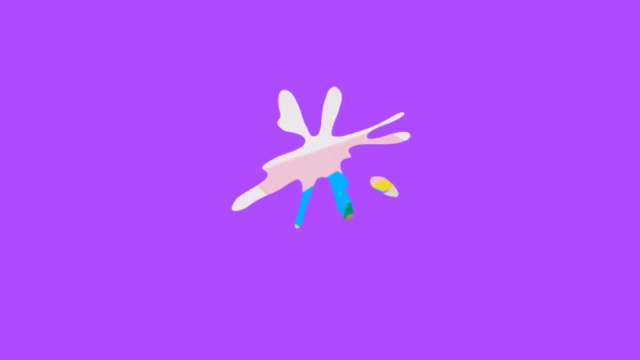 Look what a great spinning top we made. Here we go. I haven't had this much fun ever since I jump raced with the frogs back in Tibitaba. Great idea, How much longer do I have to wait? I want to jump with the frogs, Sue. 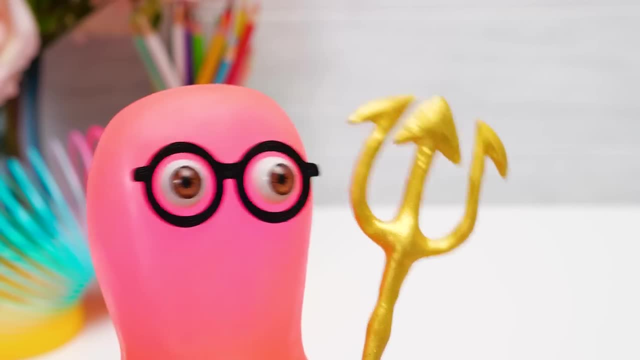 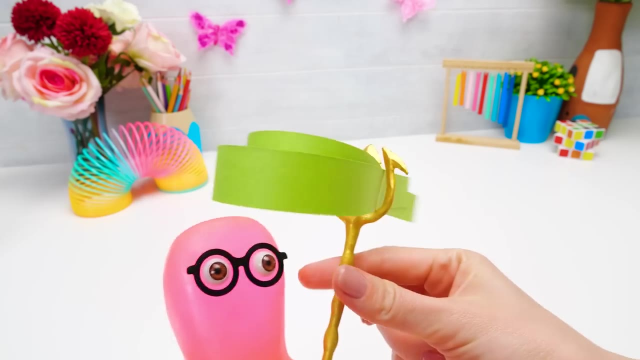 Oh, sorry, but I don't have any suitable paper left. It's a good thing there's still plenty of fish in the sea, isn't it? Here you go: One man's trash is another man's treasure. Good point, Sammy. I like your thinking. 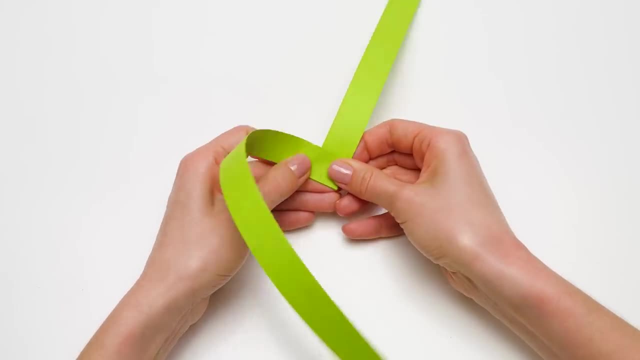 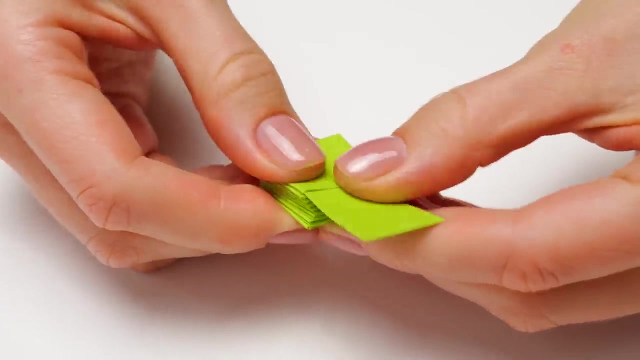 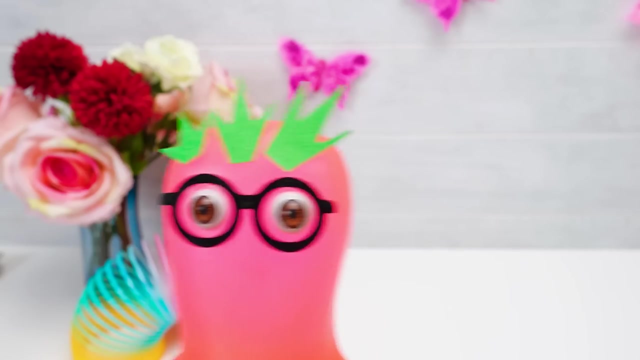 Are you ready, friends? Three, two, one, let the speed paper folding begin. So, Sammy, when did you get so wise? It's hard to stay the same after a day in the pond surrounded by frogs. Susan, Oh, wow. 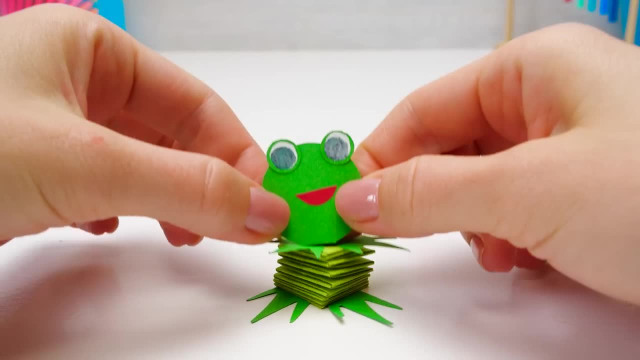 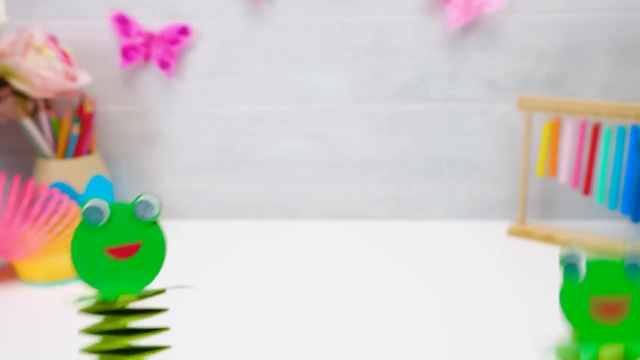 That must have been a very interesting day, And we're done here. Oh wait, Let's make our buddy a friend. Ribbit, ribbit, Jean Jacques, is that you? I missed you guys so much. Come on. 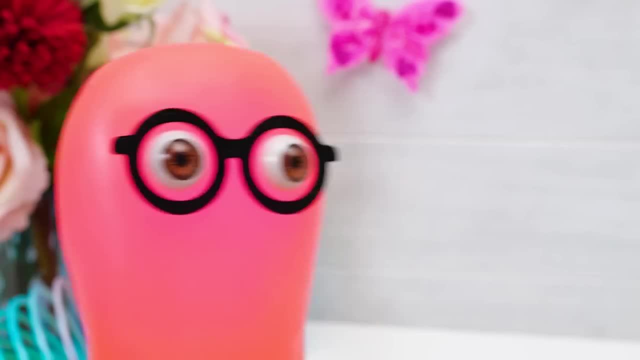 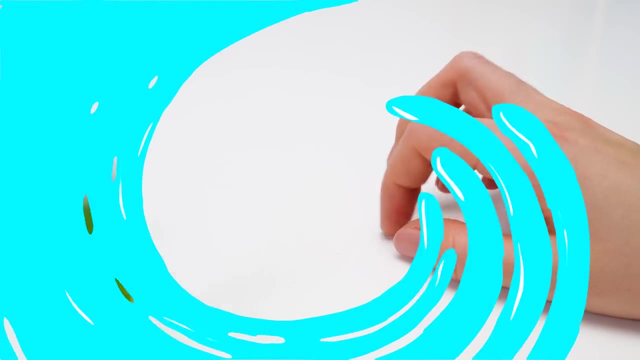 What's gotten into you? How could I forget? My frog friends were real ninjas. They even had ninja stars and stuff. No Help, Ninja stars, you say? huh, How's this for a ninja star, Sammy, You've already done it. Wow, that was fast. 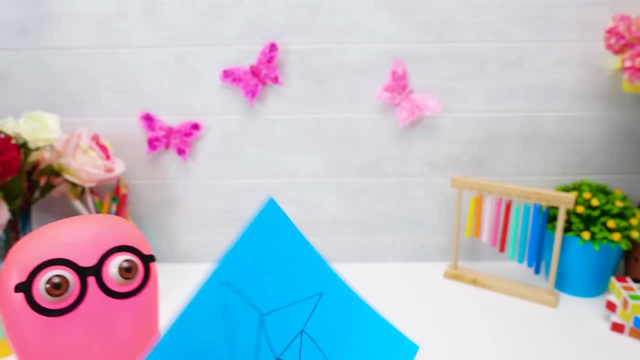 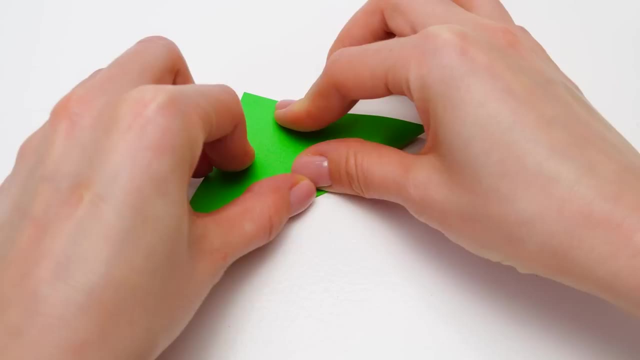 Cool, Now throw Throw Hi-ya. It doesn't work very well, Sue? Of course not, because it's just a sketch. Now I'm starting to make a ninja star. Just give me a minute, Hi-ya. 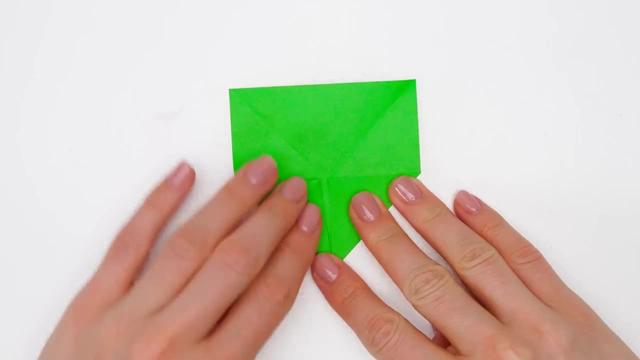 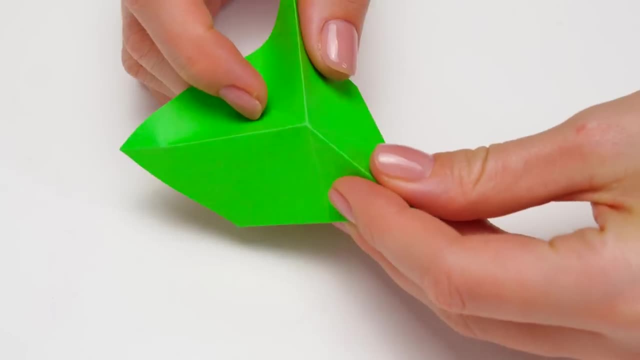 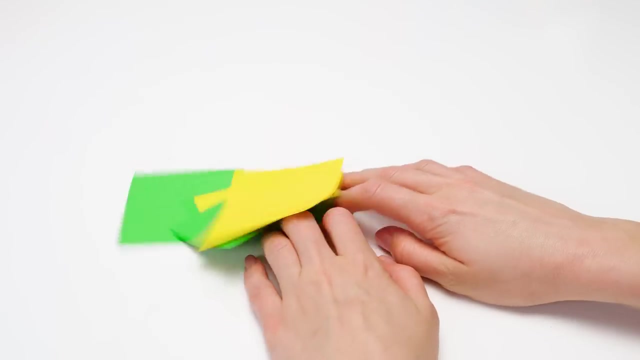 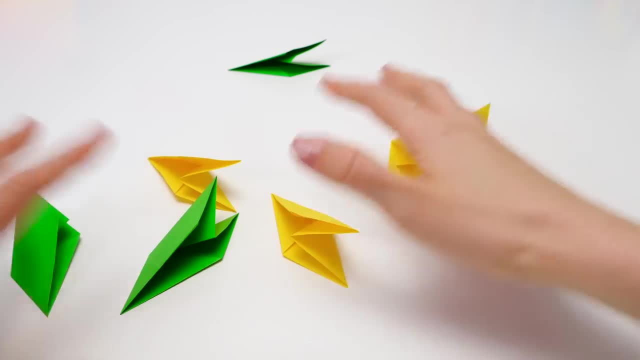 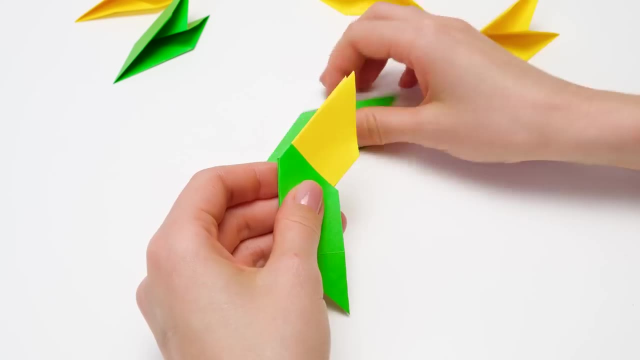 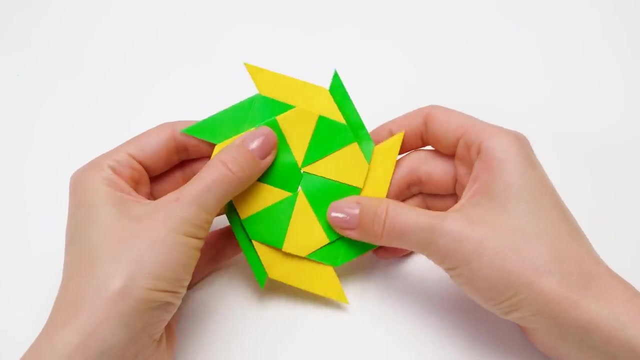 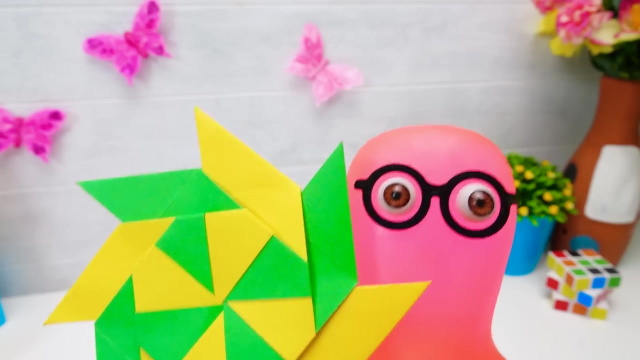 Although these pieces of paper are just what I need. Cool, Let's put it all together. This should be super cool, Sammy. catch So cool, You know. it reminds me of something. It's colorful and it's spinning. 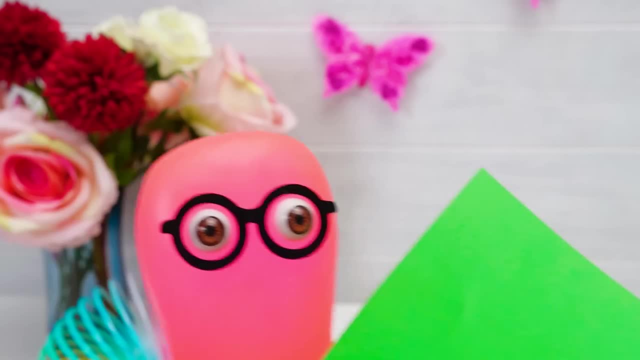 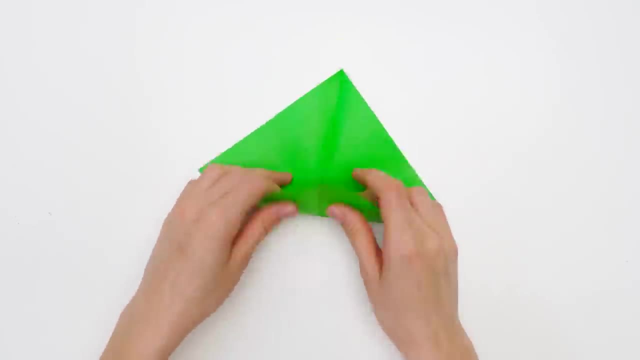 I know It looks like a spinner. Yeah, It is so great that we came up with the same idea. Tell me about it. We work like a well-oiled machine. Hi-ya, Hi-ya, Hi-ya, Hi-ya. 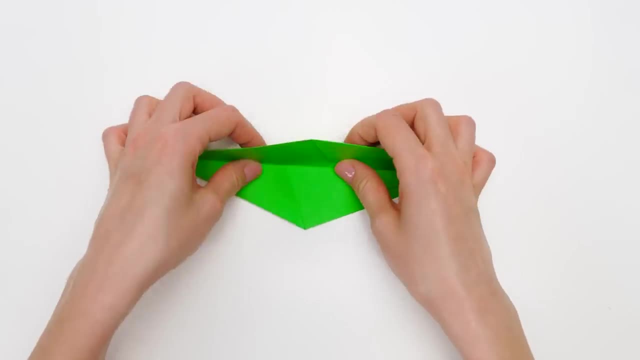 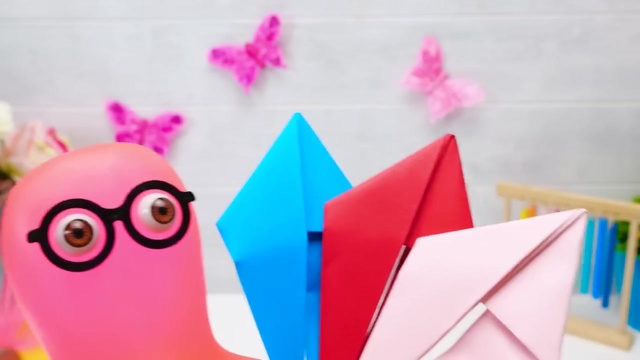 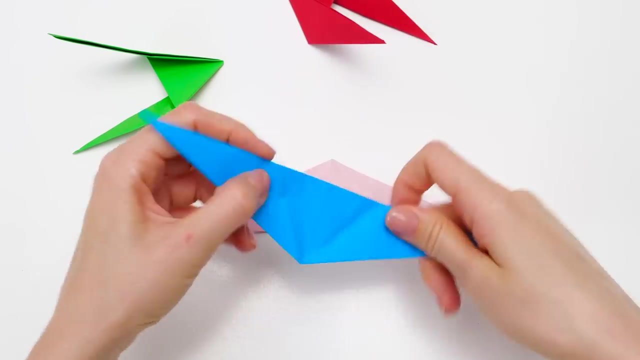 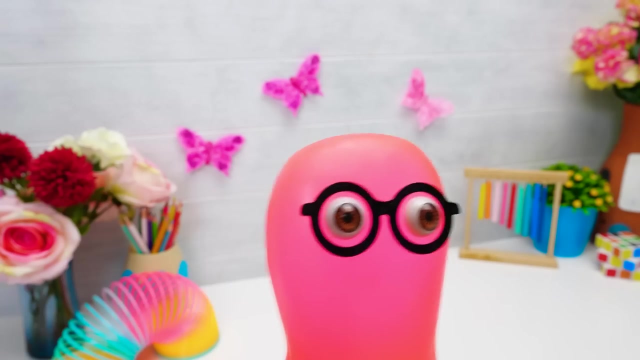 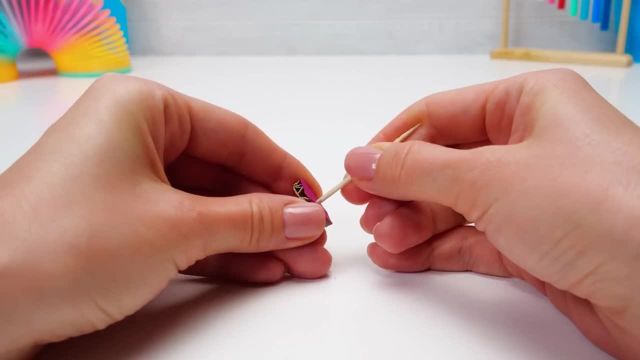 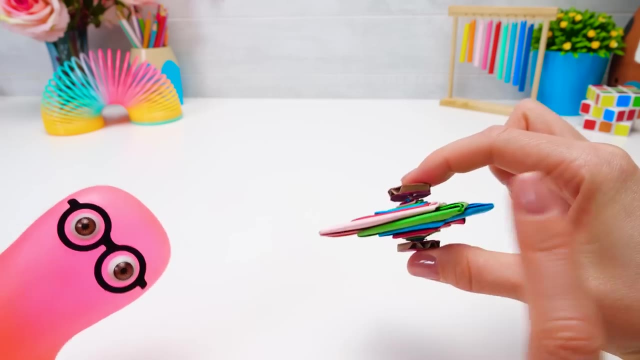 I almost got it right And look, we're nearly done here. I just need to insert the toothpick, like this, and glue two pieces of cardboard from both sides. Spin it, Sue, Spin it hard, Yay, Cool. 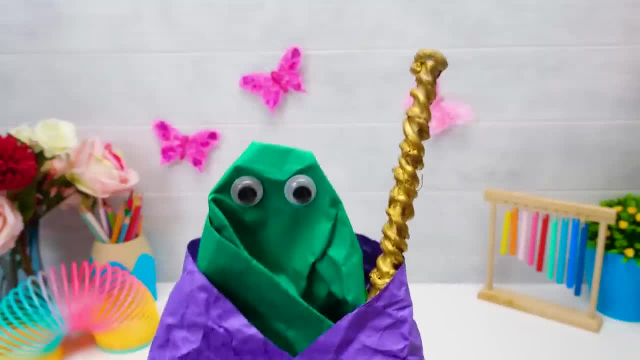 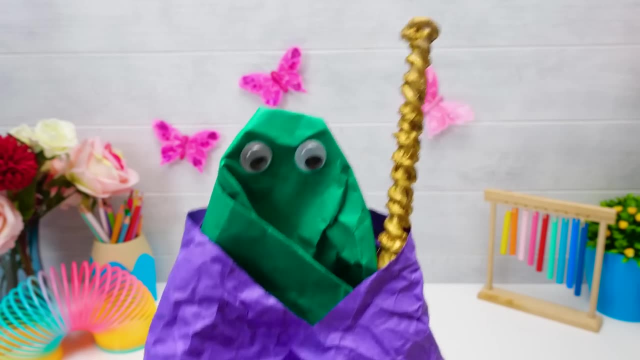 Uh-oh, I don't feel so well. Congratulations to you, Sue and Sam. You have spent so much time folding paper, you have reached a diamond level And now you'll learn about the secret. super cool origami craft. What's up? 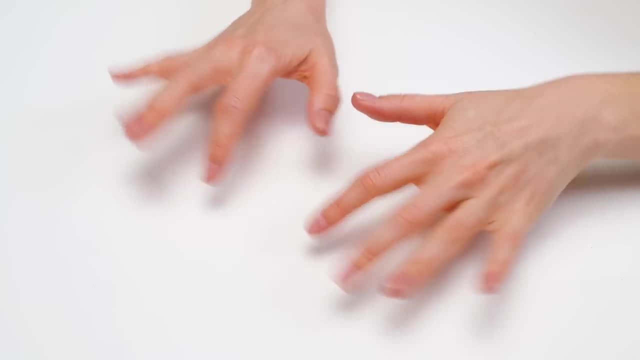 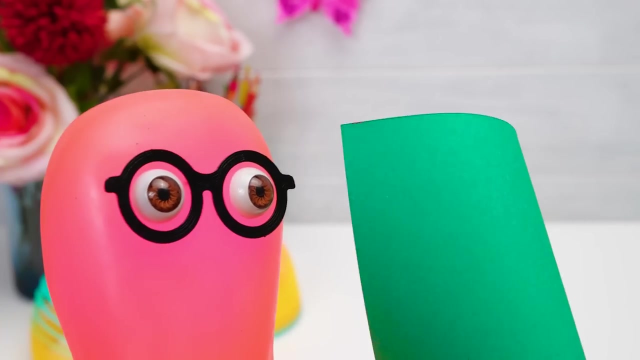 Oh, stop it. Origami Master, That tickles, Ha-ha-ha, Brr. strange. I don't know how, but I got the idea for my next craft. So what was it? This end goes here, and then this one goes where. 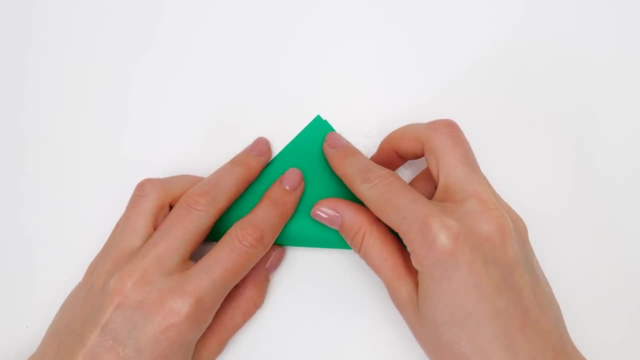 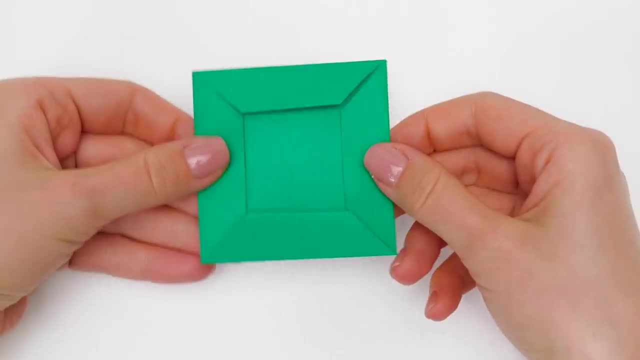 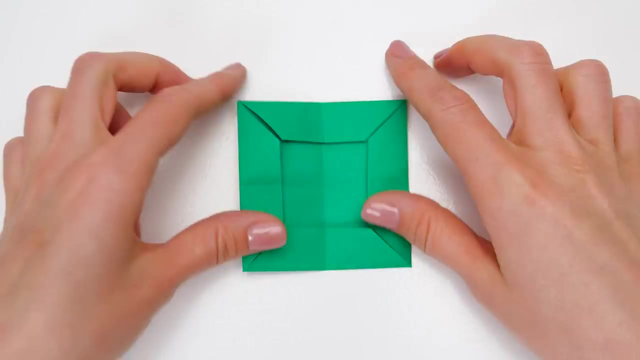 Sue, a little help. Hmm, let me see. If I remember correctly, it should go something like this: Wow, Oh yeah, that's right Now I'm starting to recollect everything. Nice, Then let's get on with it. 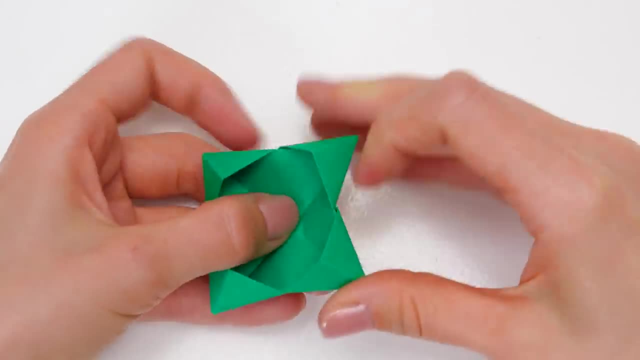 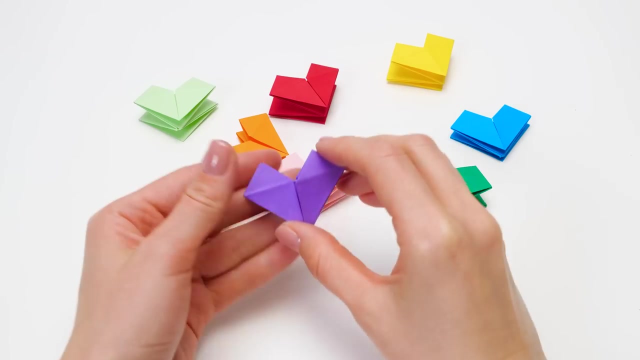 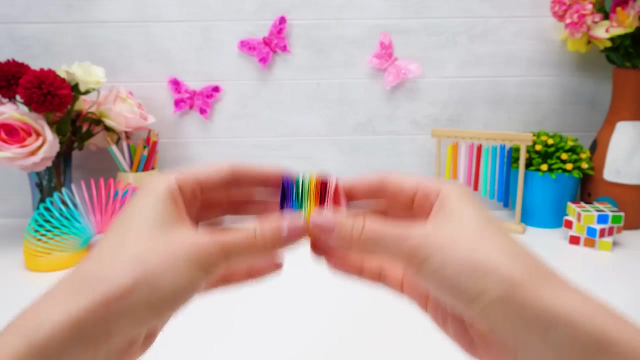 From my paper heart to yours. That's sweet, But we will play later with it. We've got a lot of steps to do. Check out this caterpillar: It's so much fun, Wow. But I feel there is one more thing. 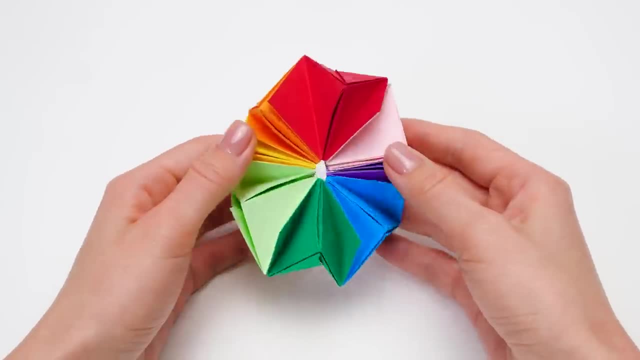 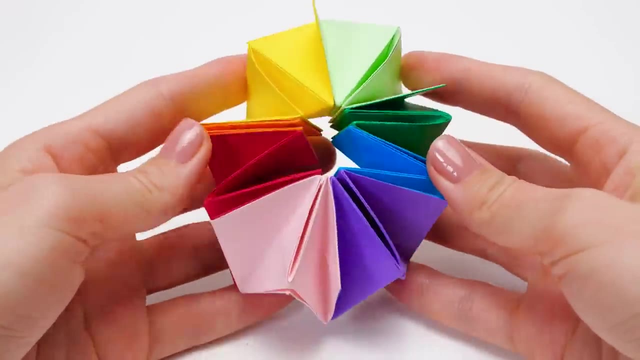 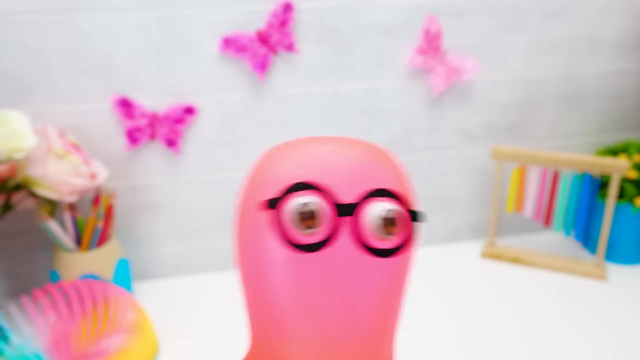 Whoa. So this is what the super secret craft is all about, What It's fun and all. but I'm getting a little tired of staring at things. I can literally feel the energy vibrating in me. Just don't tear the house down. What should I do? 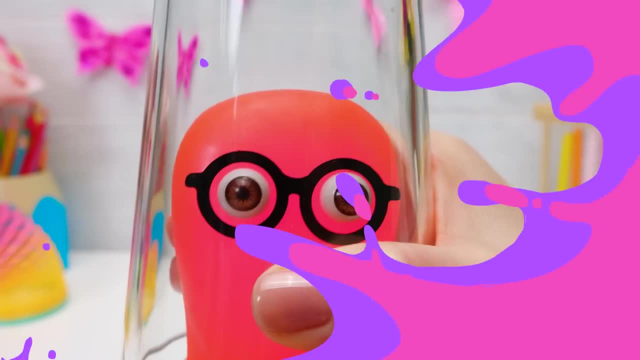 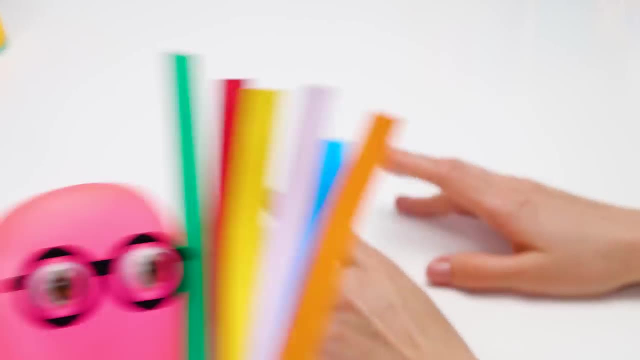 Hmm, how do you feel about soccer? Okay, Sammy, I'm gonna let you out, but you gotta use all this energy to bring me paper right. Holy cannoli. I hope he doesn't forget about the paper. What Wow. 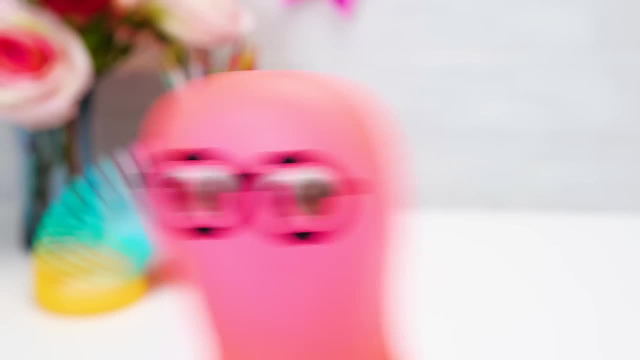 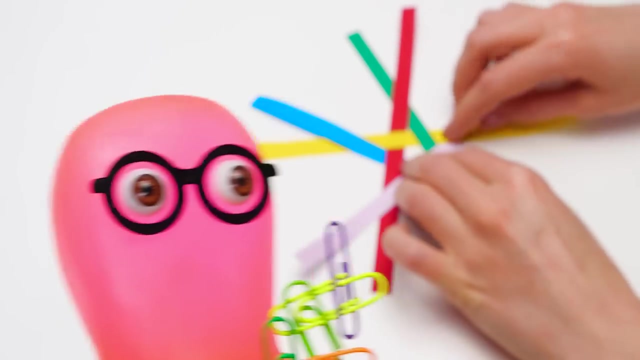 Oh, don't mind me. Just ran around the earth, Picked up some paper you asked for, Like right around the globe. you mean Wish I had a few paperclips at hand. It's already done Your paperclips, m'lady. 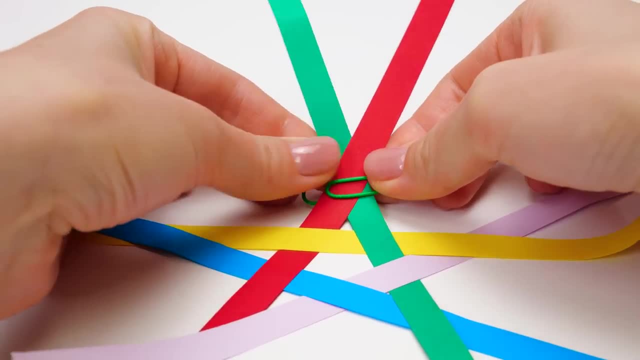 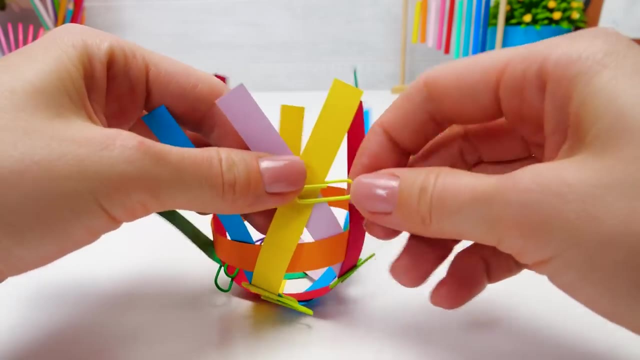 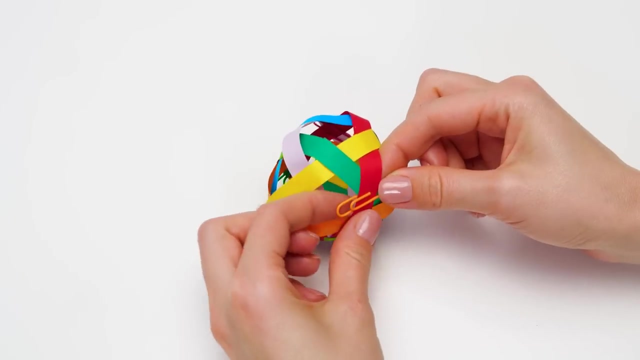 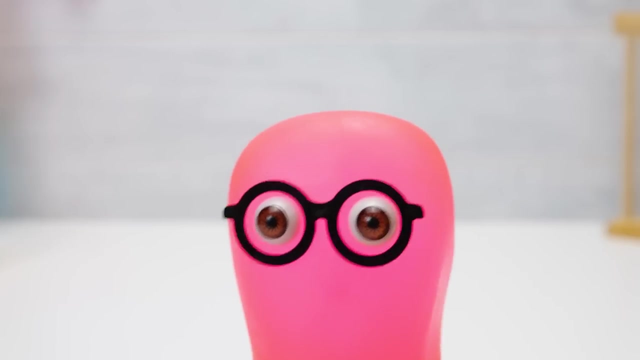 Why, thank you, But let's get back to our craft. There's a lot of weaving to be done here. Now I can remove these. Well, Is it fun, Is it a cool soccer ball or what? It's brave of you to challenge the toughest soccer player ever? 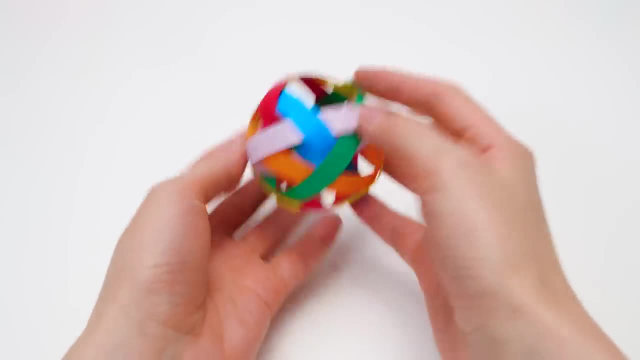 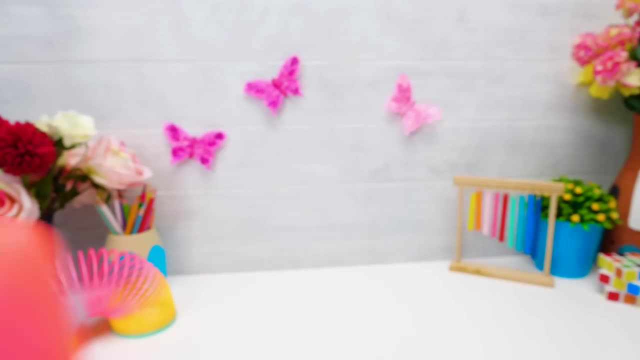 Who's the toughest player now? And since I won, the next craft will be what I want it to be. Hey, Sue, check it out. I'm like a peacock. Oh, you'll crumple them up. Aren't you forgetting something? 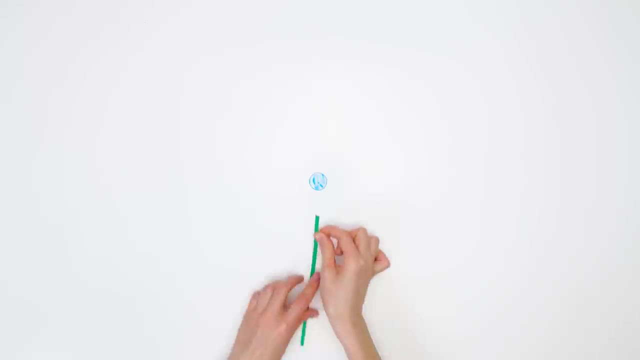 Try and catch me, Hup. As for the craft, this is where we need to glue all these elements together. As for the craft, this is where we need to glue all these elements together. As for the craft, this is where we need to glue all these elements together. 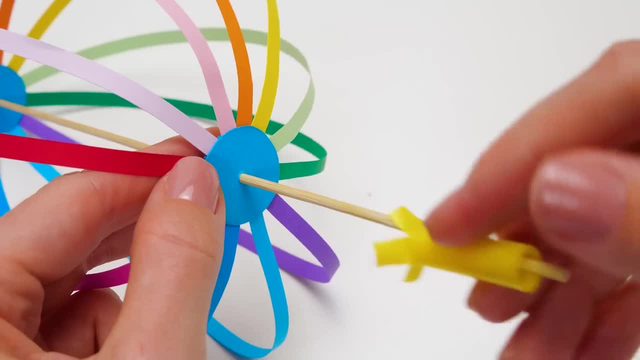 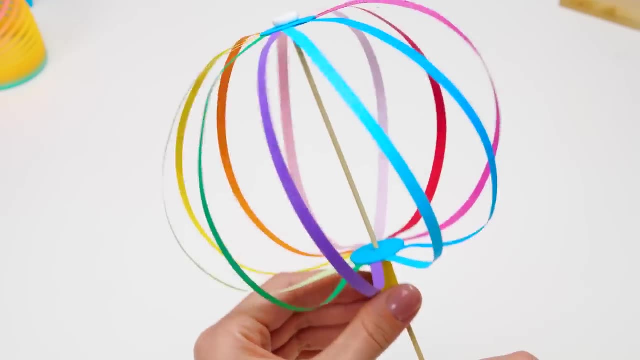 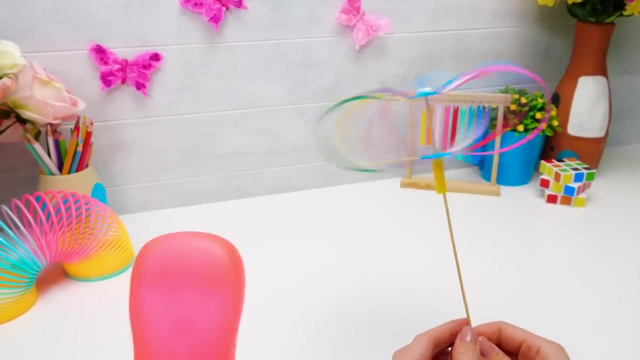 This'll make a good base. Right Now, I'm going to put all the pieces together real quick. Look at this beauty, doesn't it look cute? What is that anyway? Is it a whirlwind? Oh, you gave me a craft idea again. 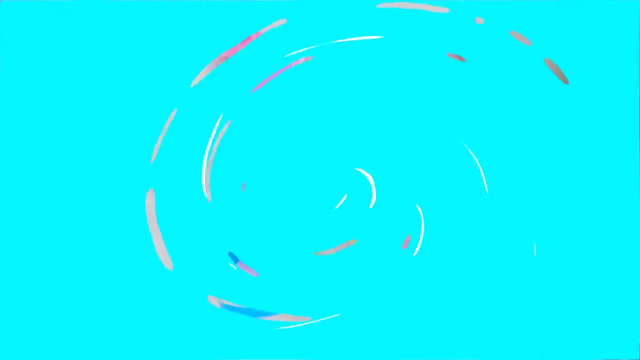 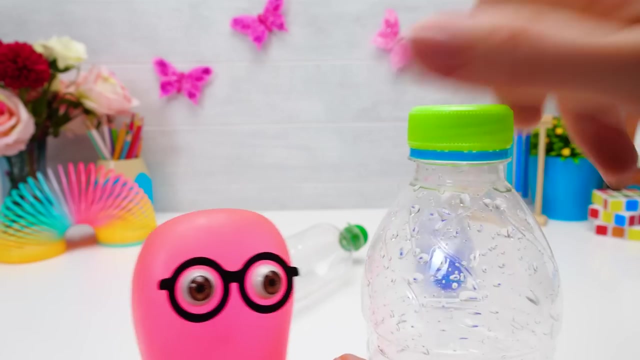 Ahaha, Uh, this is it: The things you do for a good cause. You do realize you didn't have to drink all the water to get the lids. You're kidding, right? Uh-oh, I gotta go to the bathroom. 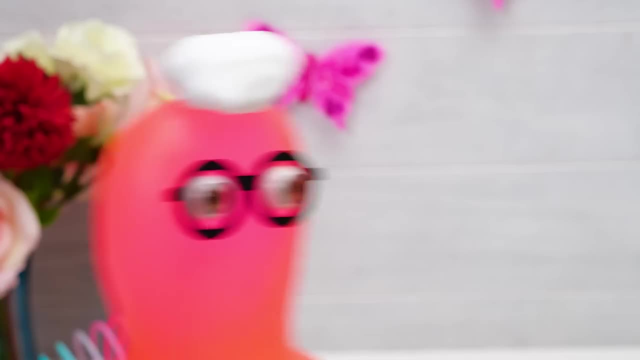 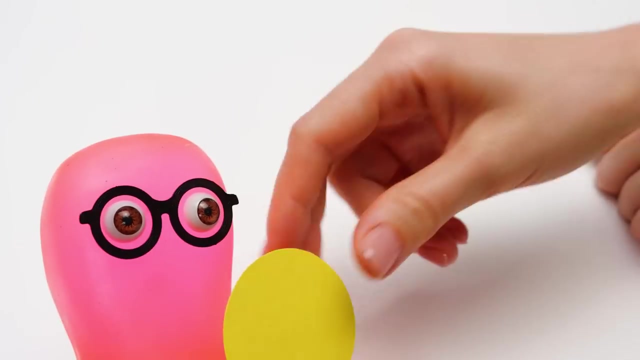 Hurry up, Oh, and grab some clay from my bag on your way out. Here you go. We'll use it to secure the stick inside our whirlwind and give it some weight. Right, I'm drawing a design on it then. 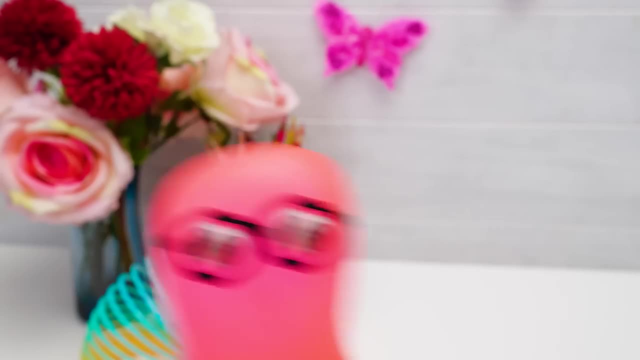 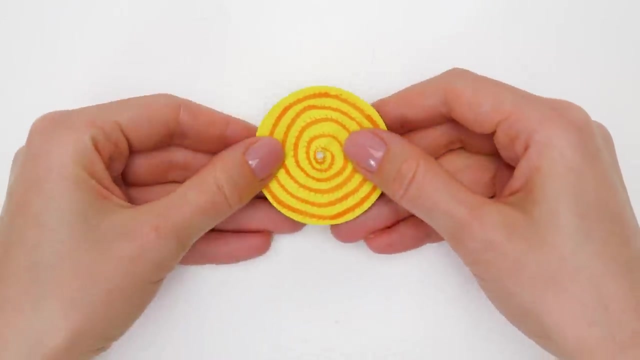 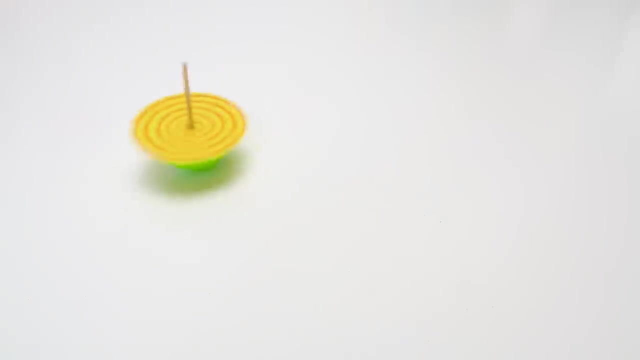 I want it to spin faster than any other whirlwind in the world. Wow, Ha-ha-ha Done, Let's see it in action. That's great. It really is the fastest whirlwind ever. Finally a problem solved.